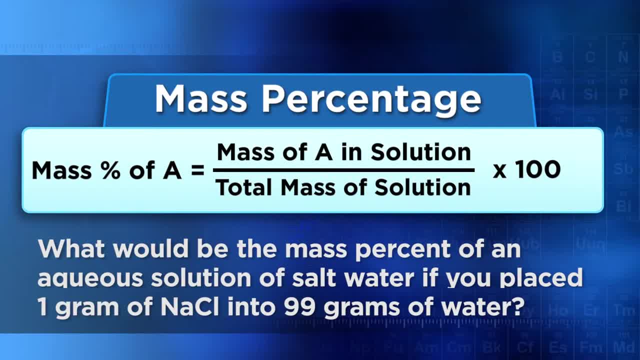 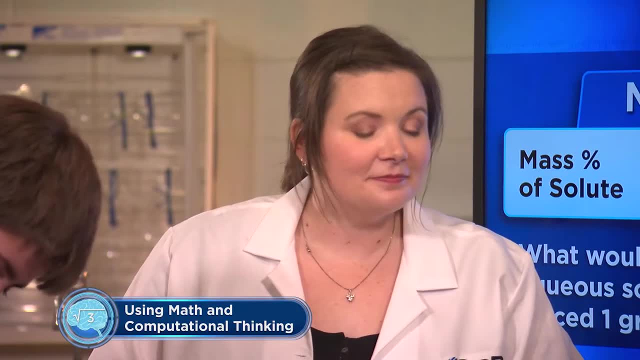 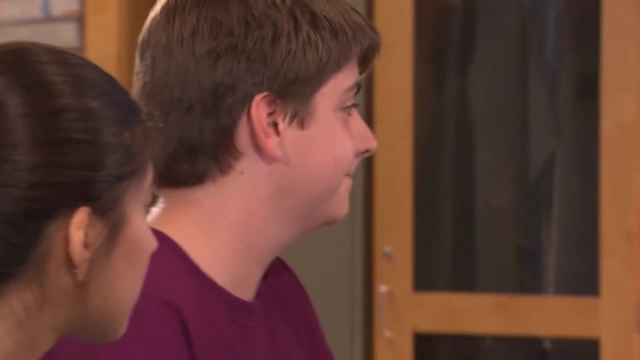 What would be the mass percent of an aqueous solution of salt water? if you place one gram of salt into 99 grams of water, Use the formula to figure out the answer: It would be one percent. That's correct. How did you get that? 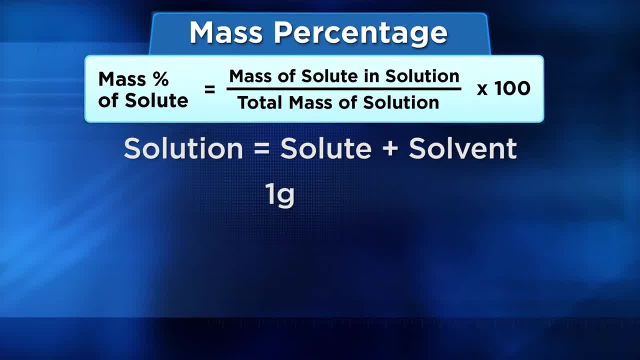 Well, since the mass of the solute is one gram, that would go into the numerator. So 100 grams would have to go into the denominator, Since that's the total mass of the solution. then divide and you get .01.. Just multiply .01 times 100 to convert it to a percentage, and that is one percent. 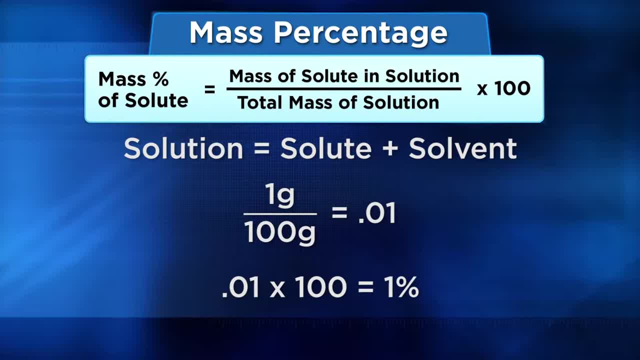 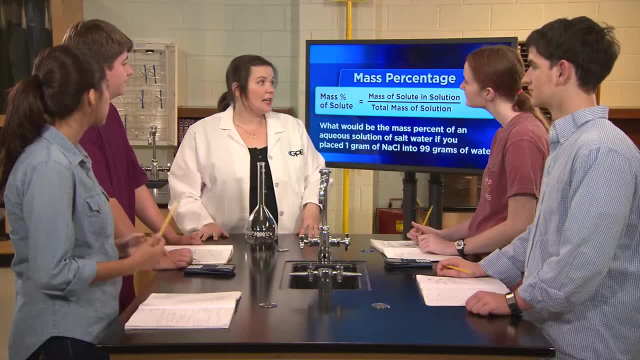 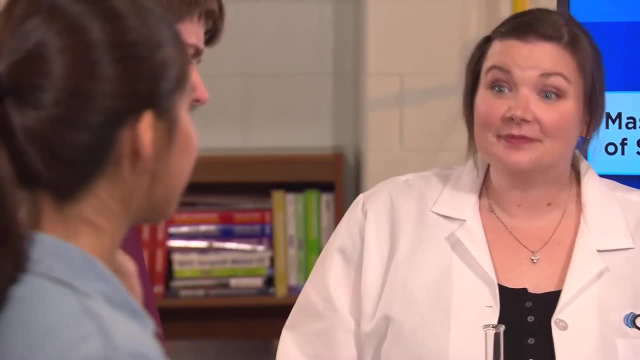 Very good, And to create a solution with a specific mass percent, the only equipment you really need is a balance of some sort and, of course, the solute and the solvent that you plan to use. Can anyone think of an example of something like this? 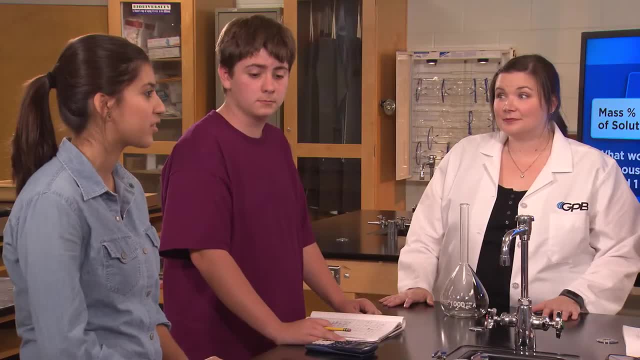 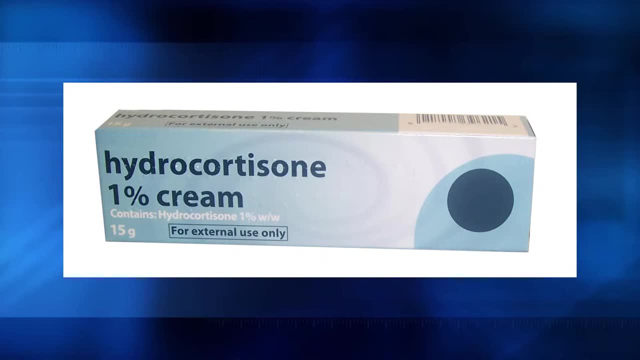 My little brother had poison ivy a few weeks ago and he used hydrocortisone cream on it. The cream had one percent on the label. Is that what you mean? That's exactly what I mean. So the active ingredient, hydrocortisone, was only one percent of the cream. 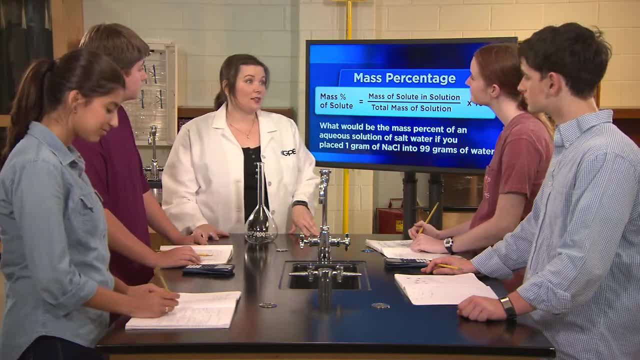 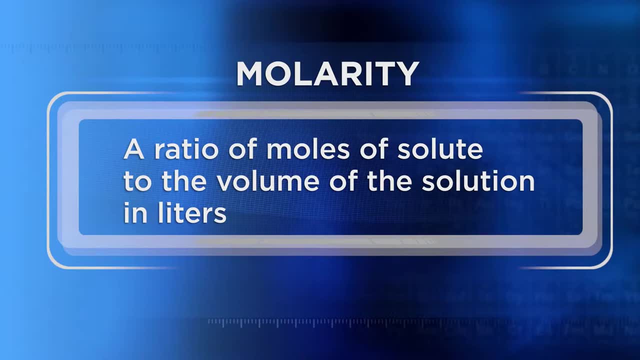 Good example. Now the next way to express how concentrated a solution is, and by far the gold standard for chemists around the world, is known as molarity. Molarity is the ratio of moles of solute to the volume of the solution in liters. 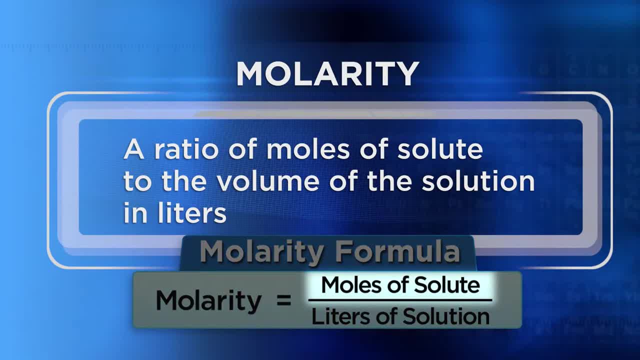 It's calculated by dividing the moles of solute in the numerator by the volume of the solution in liters. in the denominator, Molarity is abbreviated with a capital, M. A key point to notice here is the use of liters in the denominator. Since we want to measure the volume of the entire solution, special glassware is used. 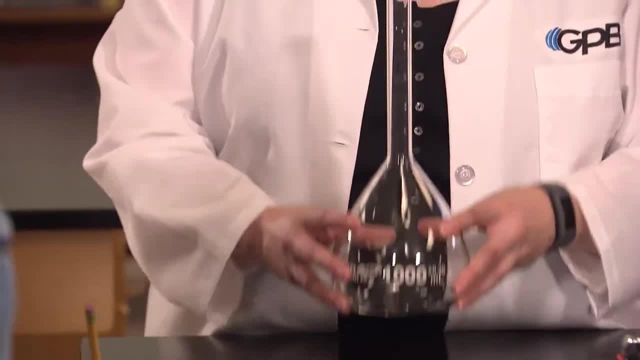 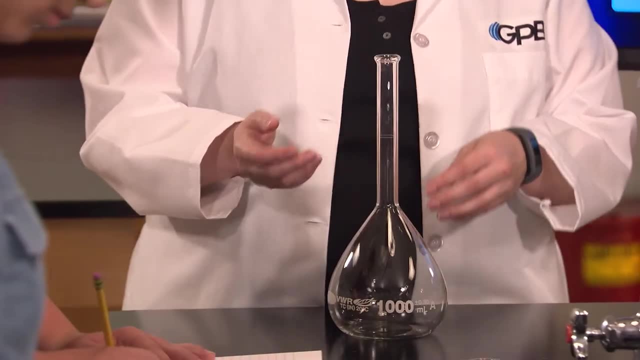 to create solutions of no molarities. A volumetric flask like the one I'm holding will allow you to put the number of moles of the solute in the flask first, then add distilled water up to the line. So now what I'd like for you guys to do is to create a solution of no molarities. 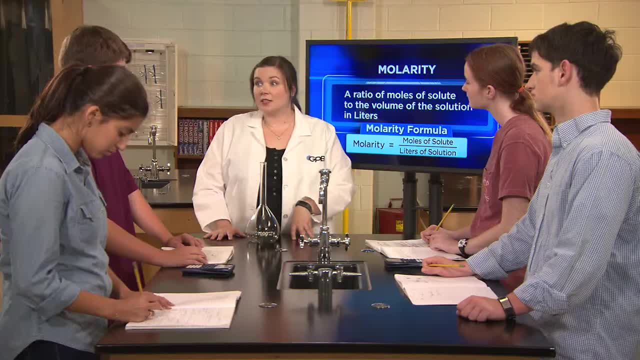 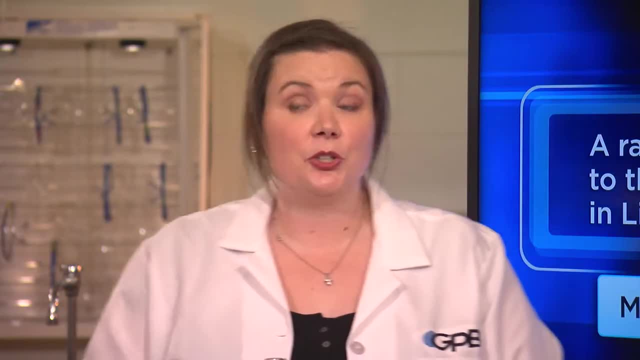 I'm going to show you how to do that. The first step is to create your own solutions of no molarity. Team 1 should create 500 milliliters of a 1 molar copper 2 nitrate solution. Team 2 will make 1 liter of a 1 molar copper 2 nitrate solution. 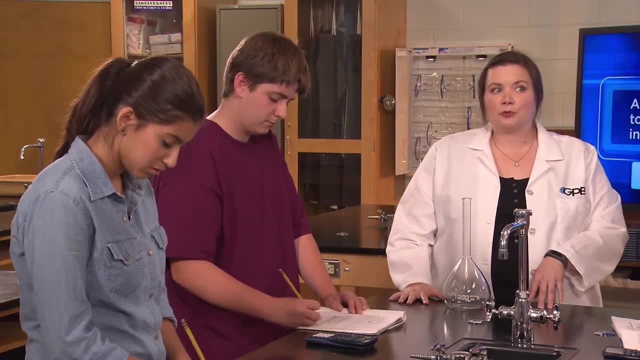 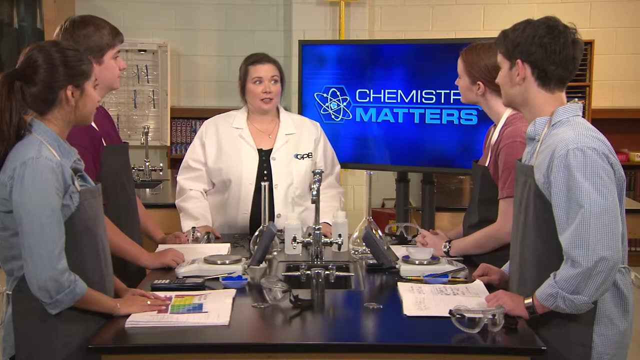 Come up with your procedures first and let's discuss them. Once I approve your procedures, you can make your solutions. Okay, everyone who's ready to present the plan that they're going to use to create their solution, We'll give it a try. 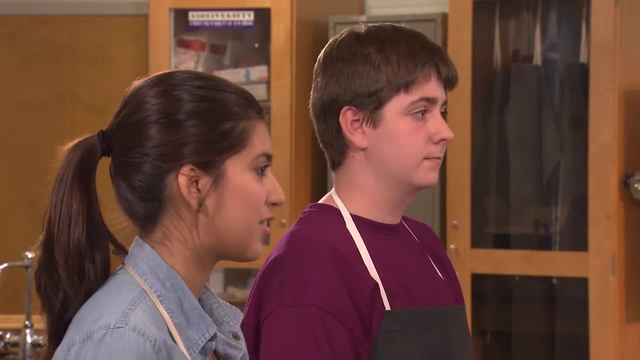 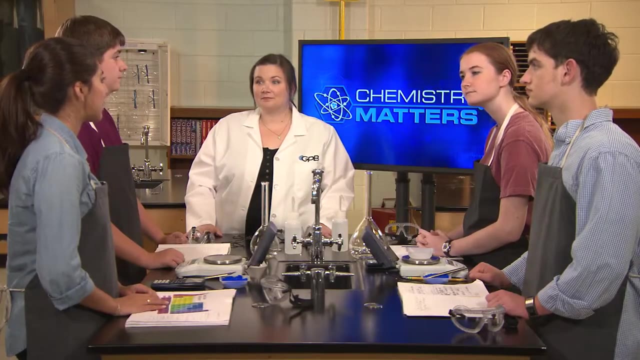 We have to make 500 milliliters of a 1 molar copper 2 nitrate solution, which means we actually need to have 0.5 moles of copper 2 nitrate dissolved in a total of 500 milliliters. of solution, right, Since molarity is the ratio of moles to 1 liter, we figured that to make a half a liter of 1 molar solution we would need half of a mole of copper 2 nitrate. That's right. 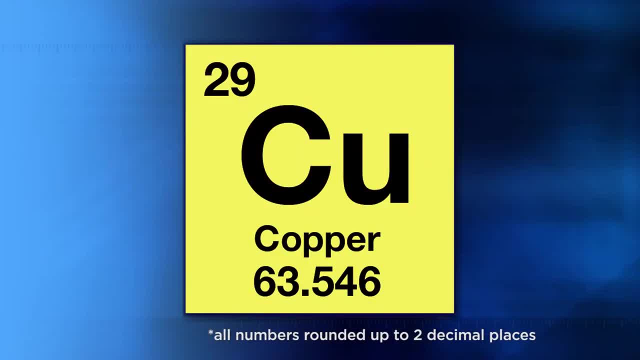 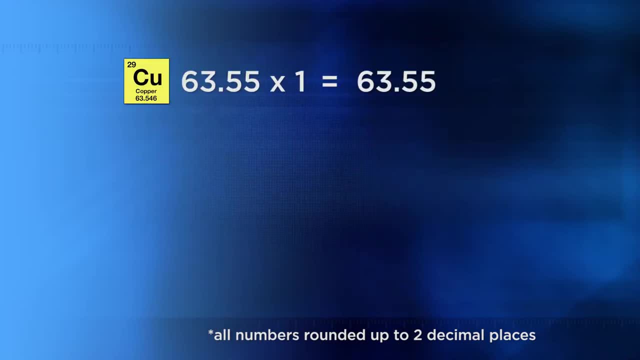 Looking at the molar masses from the periodic table, copper 2 nitrate has copper with a molar mass of 63.55 grams. That's right. We multiply that by 1 because there's only 1 copper in the formula. 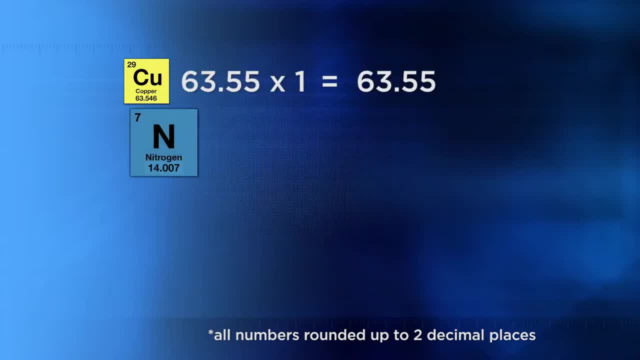 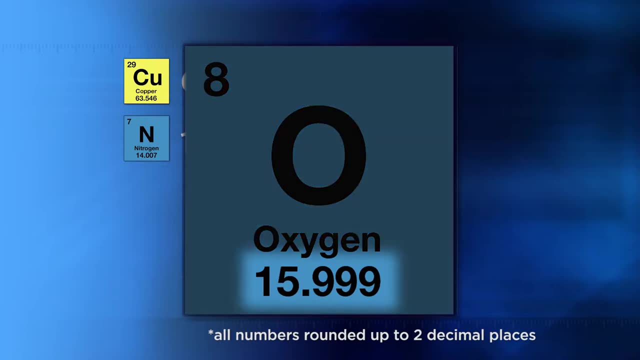 Nitrogen has a molar mass of 14.01 grams, And because copper 2 nitrate has 2 nitrogens in the formula, we multiply that by 2. And oxygen's molar mass is 16.00 grams. 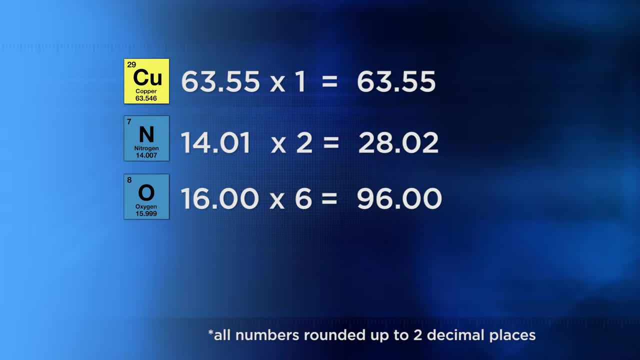 And we multiply that by 6 because copper 2 nitrate contains 6 oxygens in the formula. After multiplying all of those and adding them up, 1 mole of copper 2 nitrate would have a mass of 187.57 grams. 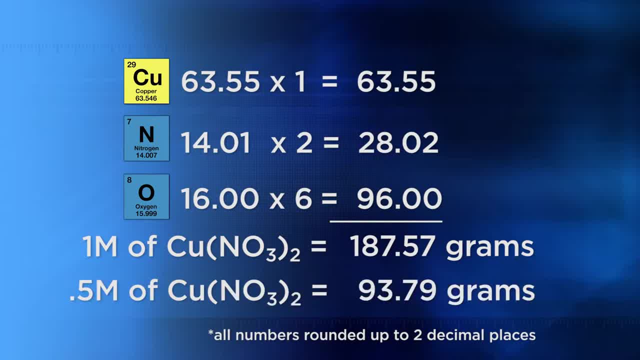 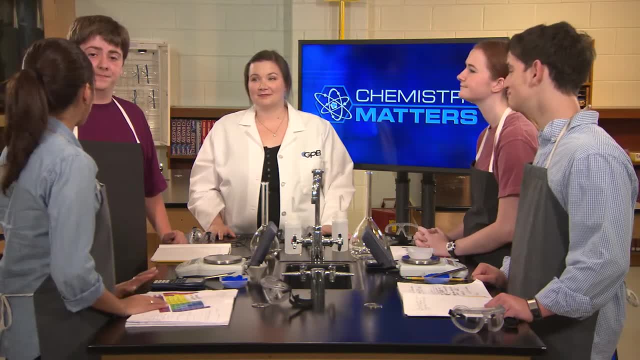 Okay, So half a mole would be 93.79 grams. So now we just add that to the flask and add about 500 milliliters of water in there. Wait, Actually, I think we just put the copper 2 nitrate in and then add water until it comes. 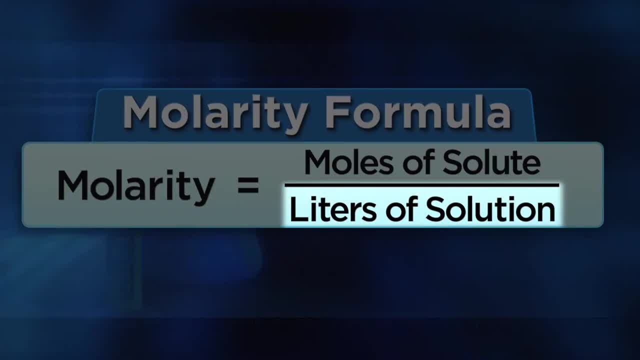 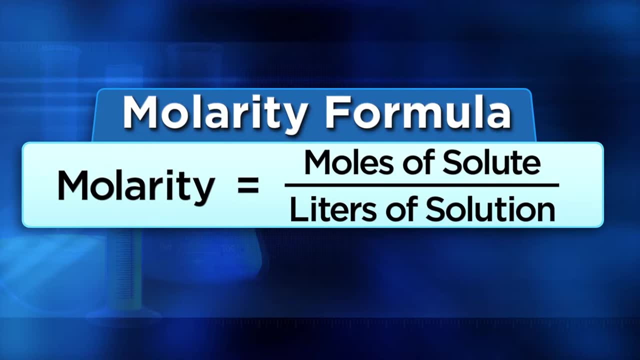 up to the 500 millimeter mark. Oh right, The denominator has liters of solution, not just solvent. Yeah, The copper 2 nitrate is going to take up space, which is why we have to use this flask, I guess. 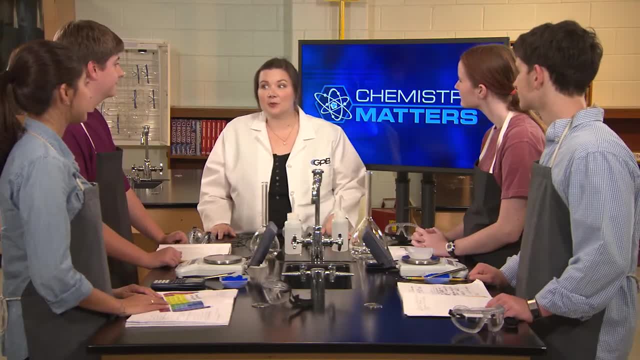 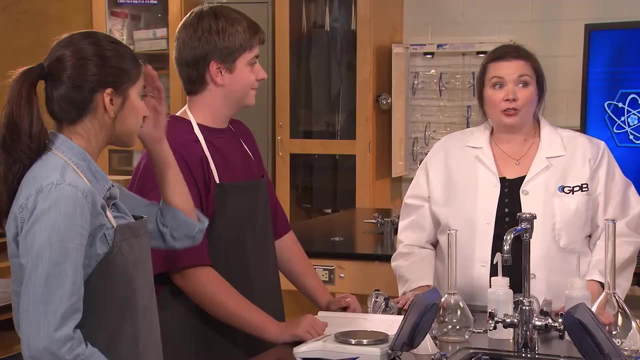 Great catch. And you're exactly right. We have to create these solutions with specific types of glassware. We have to be able to account for the volume or the space that the solute is going to take up. Your team is good to go. 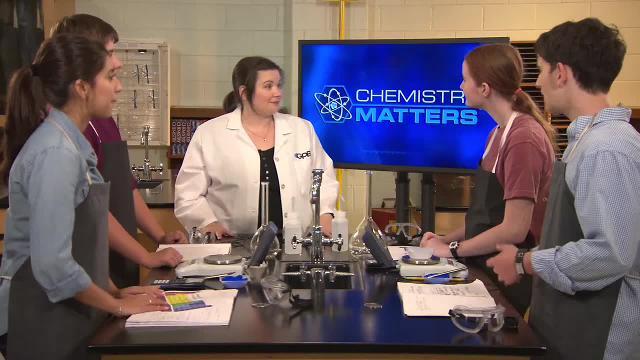 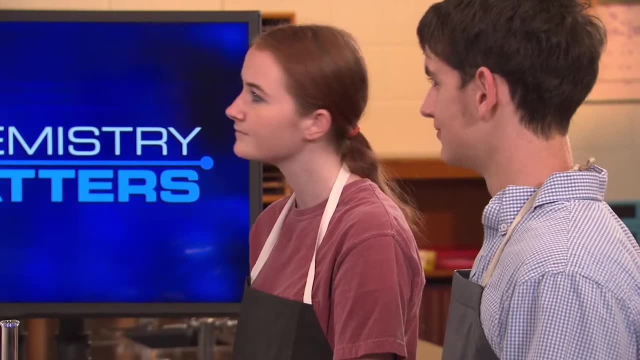 Okay, Team 2, are you ready to tell me with your plan? I'm pretty sure we are. We need to make 1 molar solution of copper 2 nitrate, which is 1 mole of copper 2 nitrate dissolved. 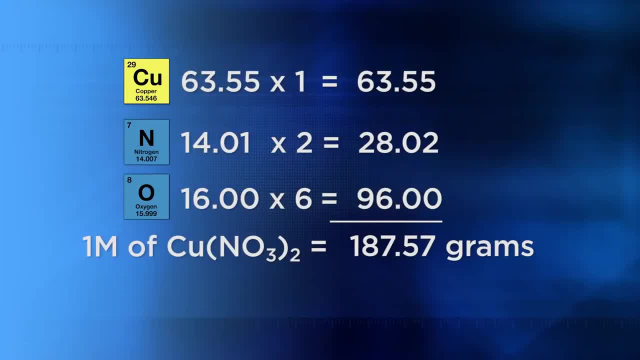 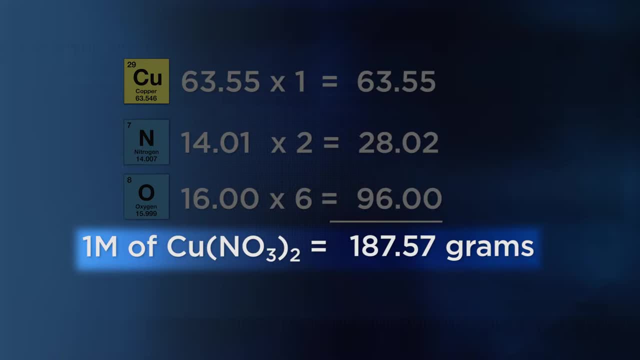 Yeah, And according to the masses on the periodic table, the molar mass of copper 2 nitrate is 187.57 grams. Exactly Yeah. So we need to mass that out and place it into the volumetric flask, right? 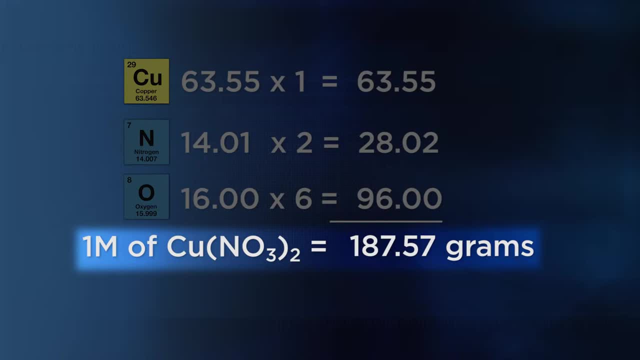 And then we'll add water up to the 1 liter mark to make sure it's 1 mole per 1 liter of solution. That sounds like a great plan. So everyone put on your safety goggles and you can all go ahead and start creating. 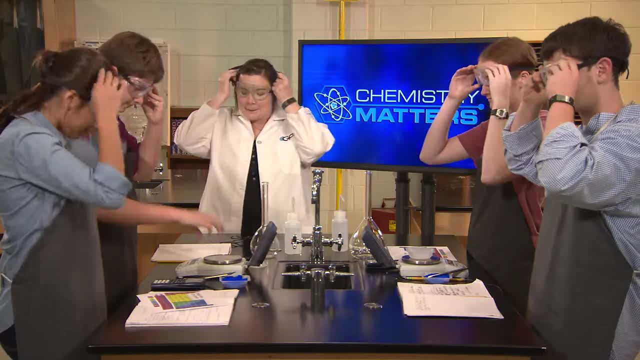 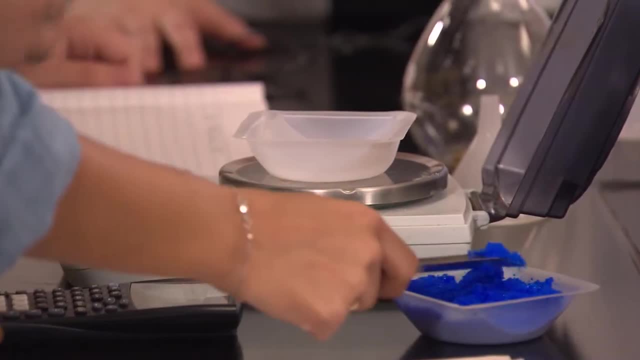 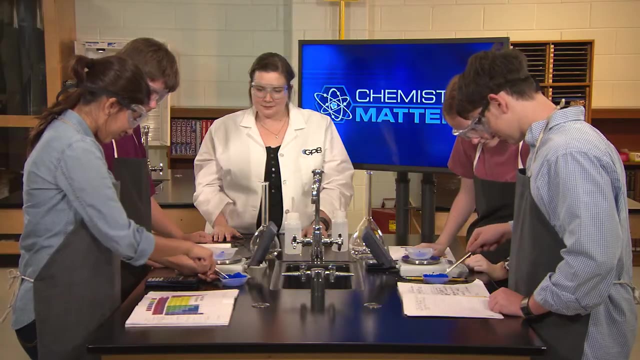 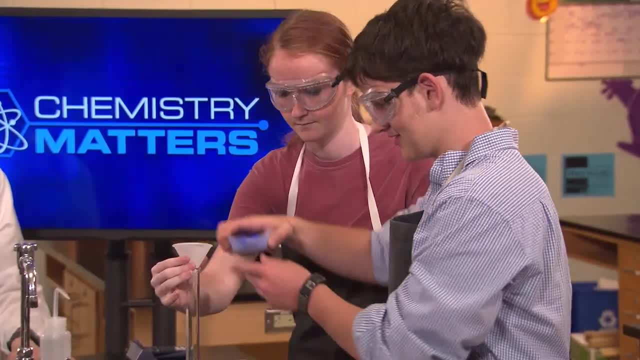 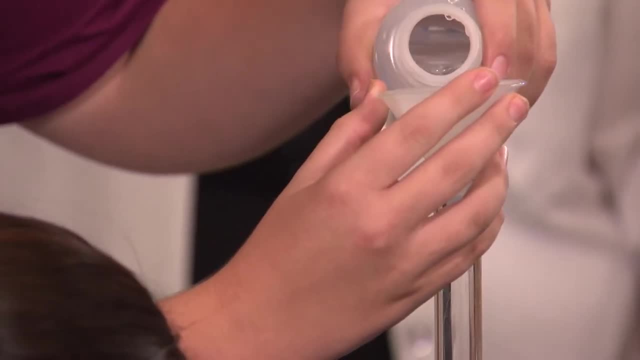 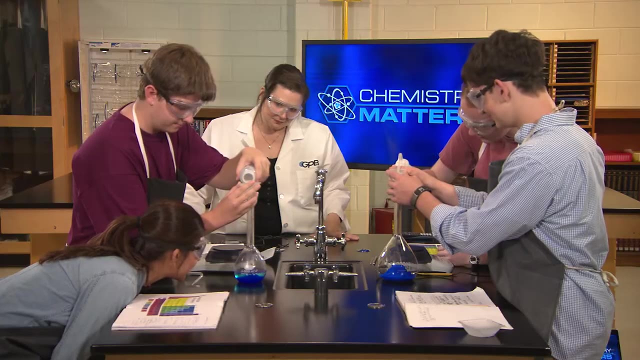 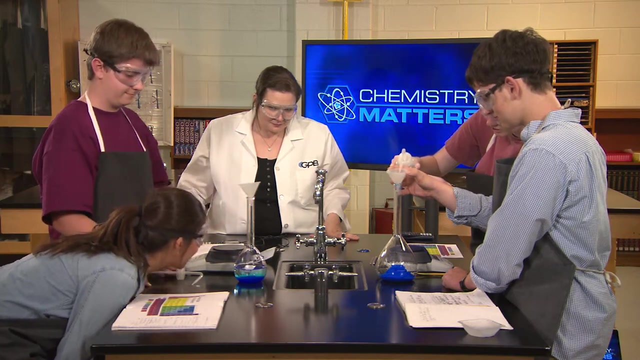 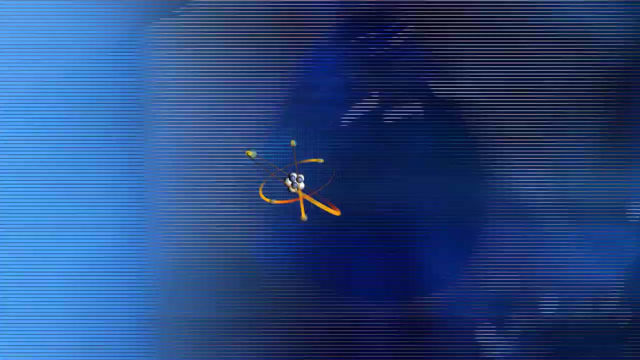 Okay, Okay, Okay, Okay, Go forward. Careful, Keep it going. That wasn't actually kind of easy. Yeah, I don't think we were Pretty cool. Okay, Okay, Okay. Whoa, Our students already described their very detailed plans for you making your job a. 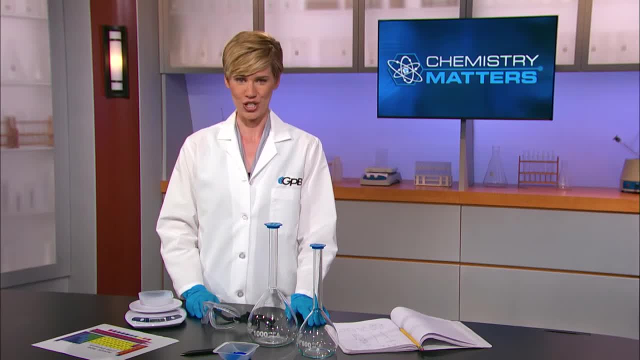 little bit easier, But you've still got the activity itself to do. By the way, depending on how you round off your atomic mass, your exact numbers could be a little different from those of our students. We'll take a break here. When you're done with the Molarity Lab, you can compare your results with the results. 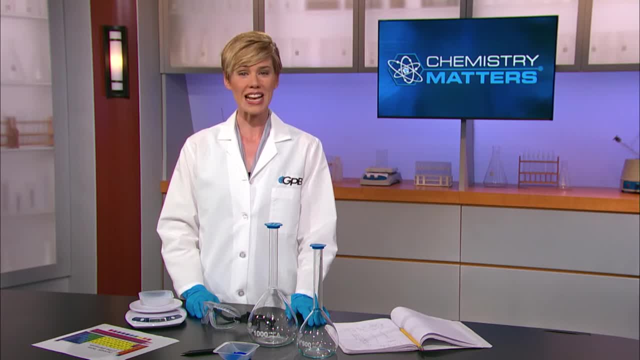 of our students. We'll take a look at those at the top of the next video on the playlist. I'll see you there, Thank you.